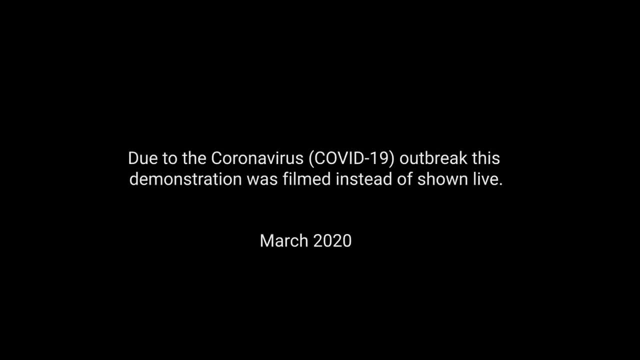 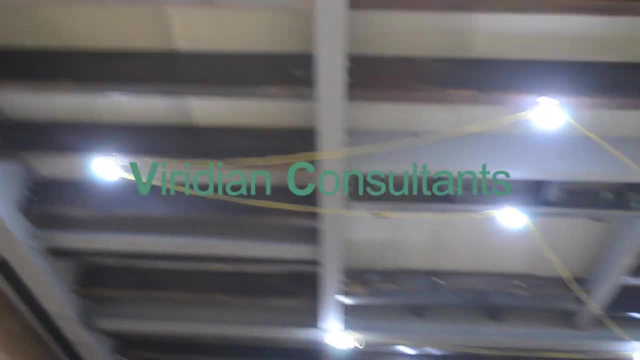 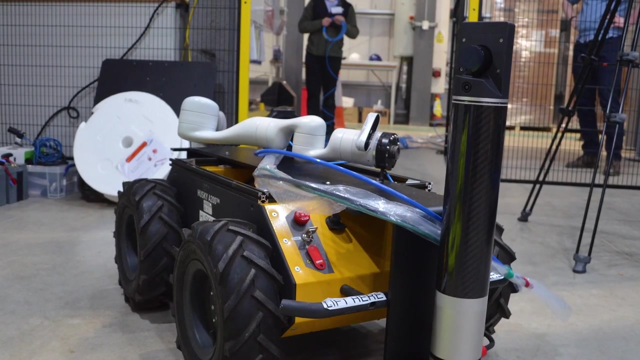 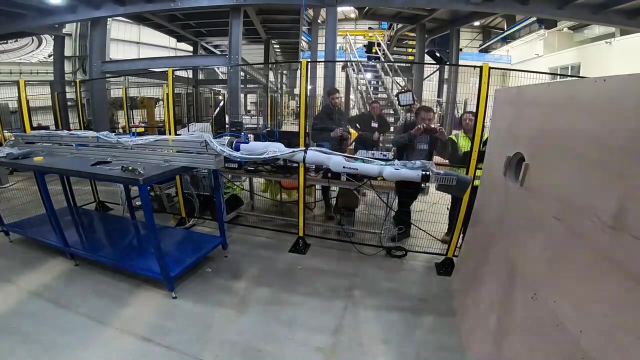 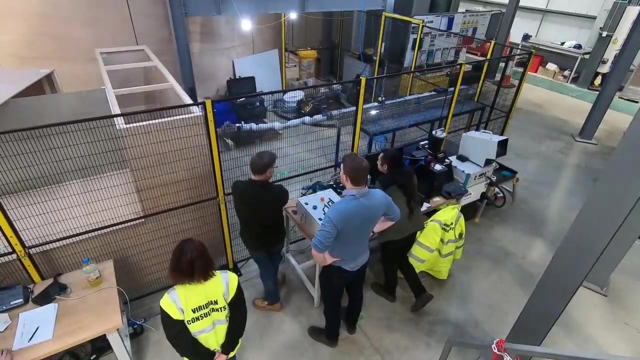 Reach seeks to demonstrate radiological characterisation sensors and how they can be deployed by a variety of different robotic systems to help users understand the environment. There's a constant requirement in civil nuclear to characterise the environment in areas where human access is not possible, getting information to make better decommissioning decisions. 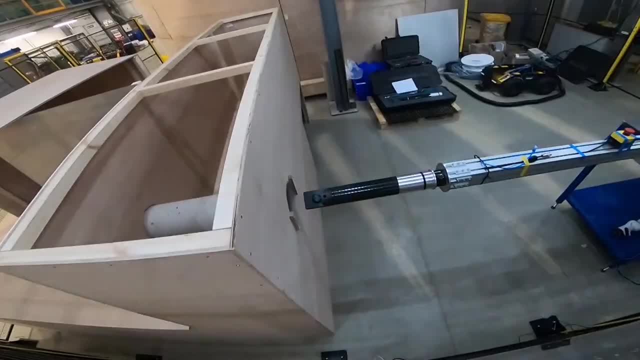 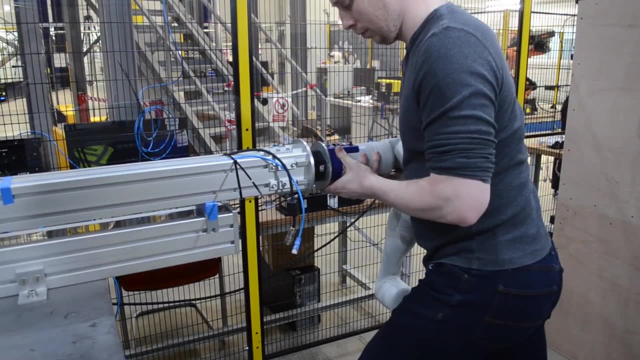 The tools developed are able to pass through small openings to enter cells and glove boxes to determine the source of radiometric dose. To aid this, we have developed another robust and universal interfacing system to enable quick and effortless swapping of tools while wearing protective equipment. 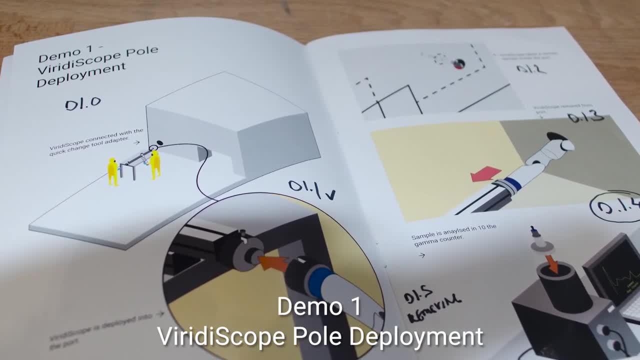 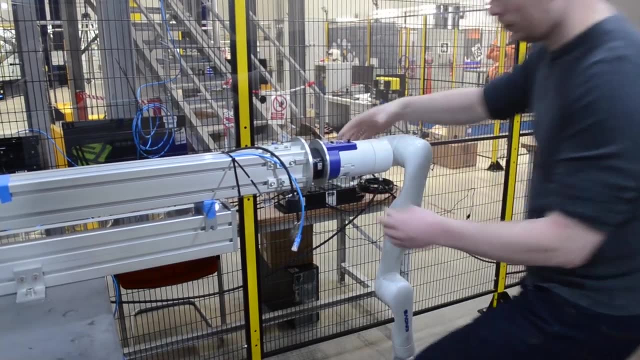 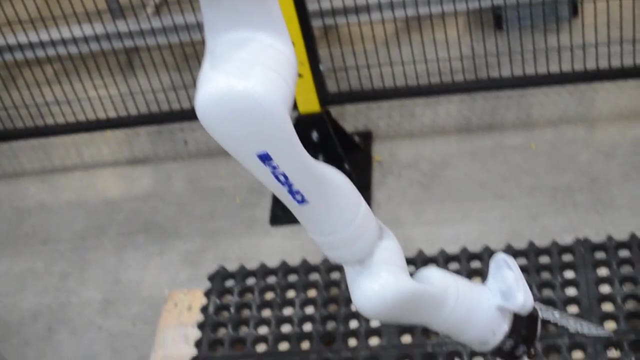 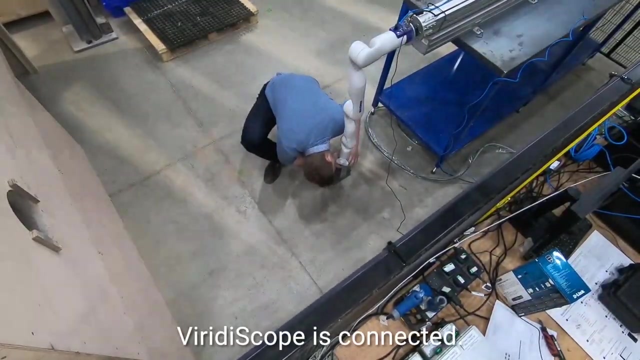 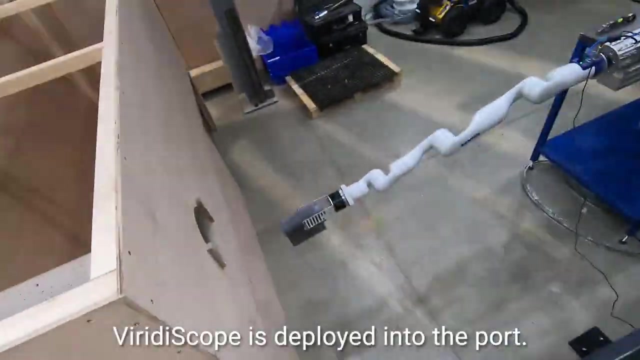 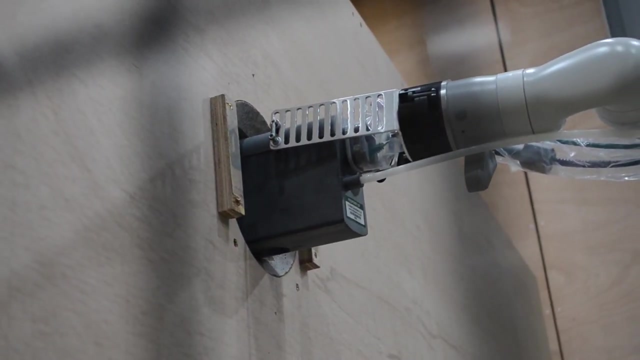 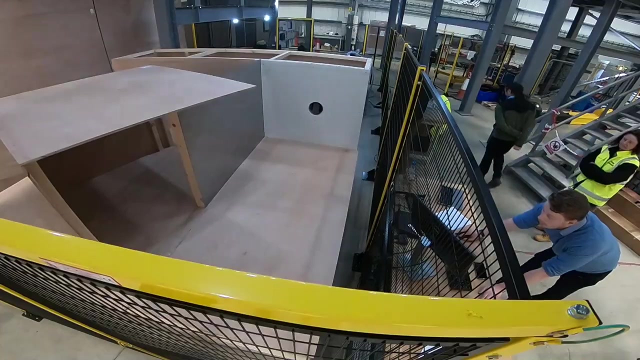 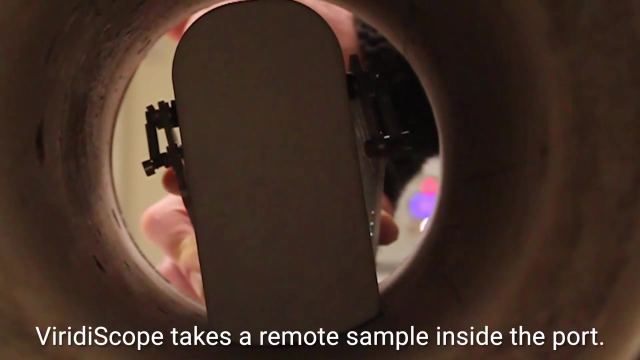 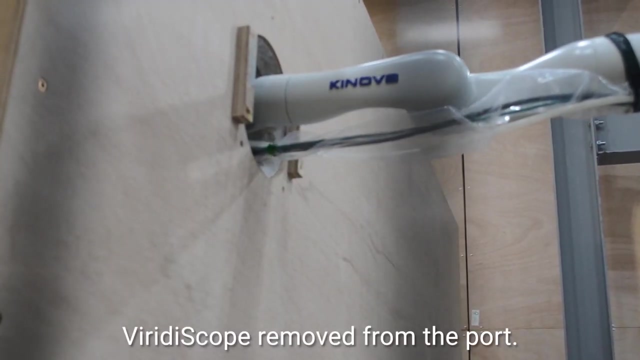 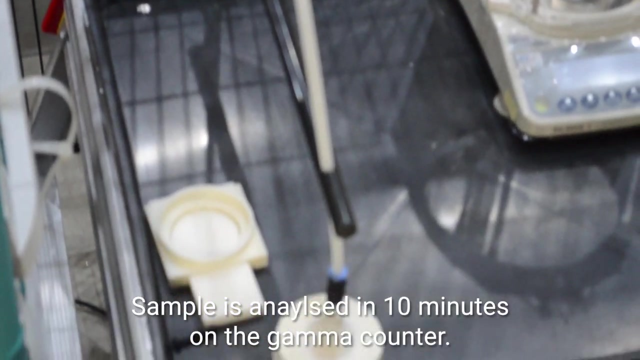 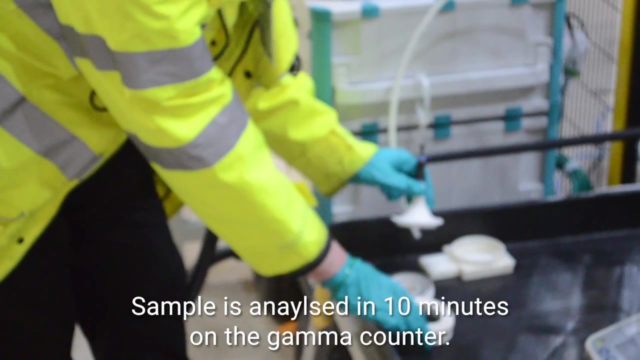 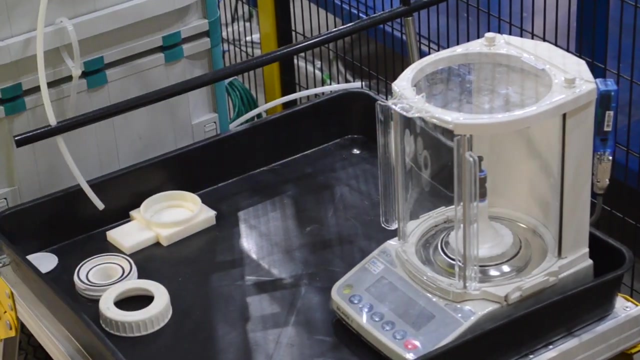 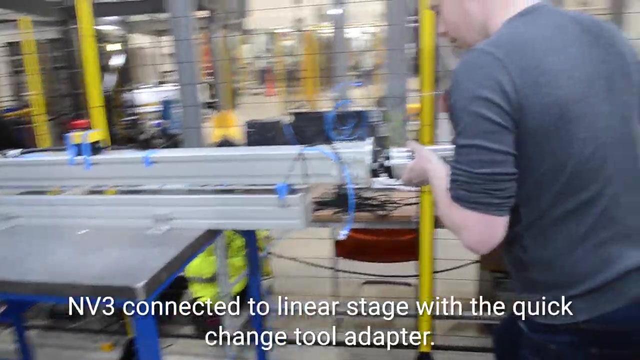 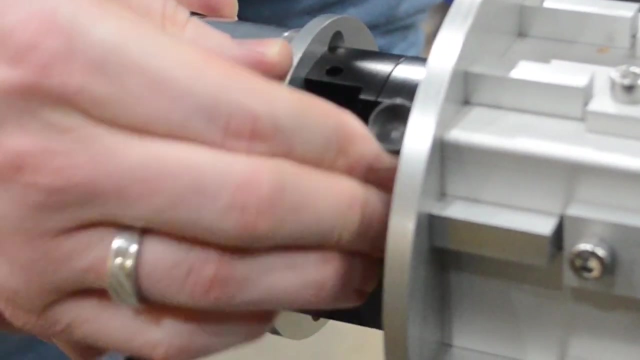 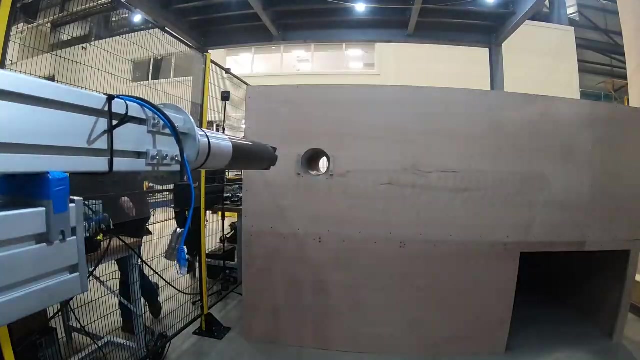 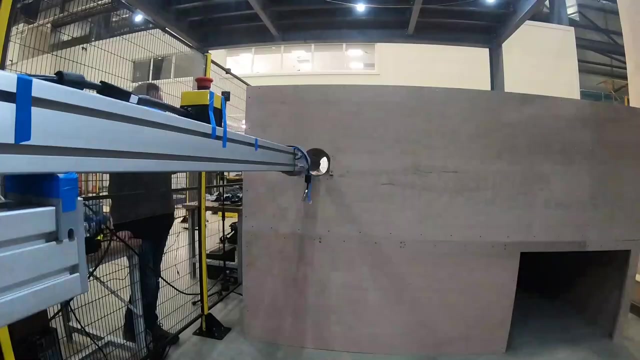 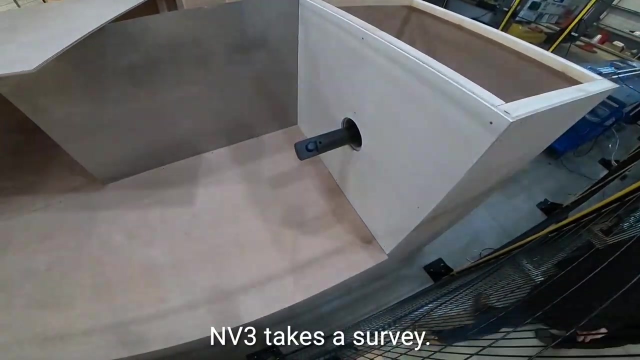 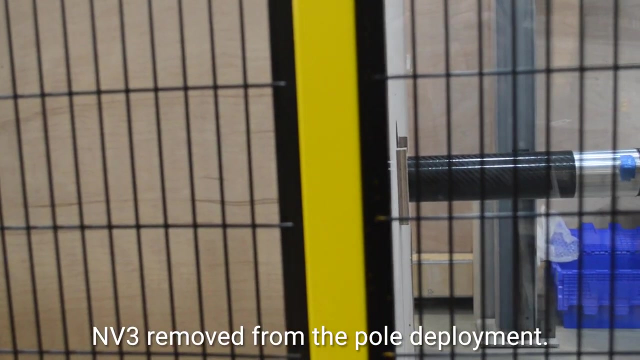 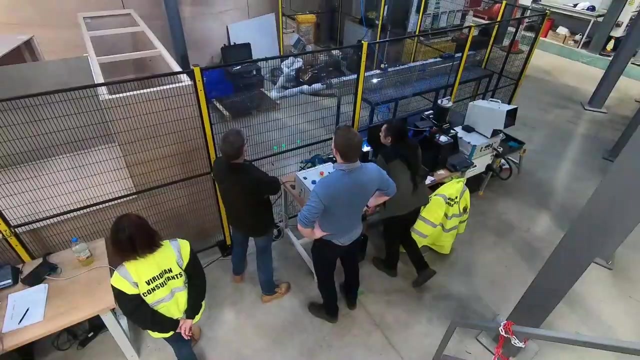